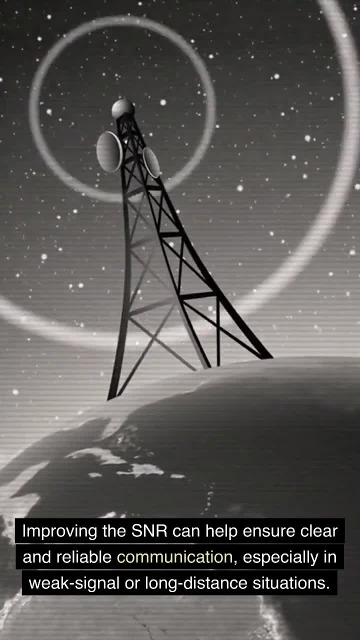 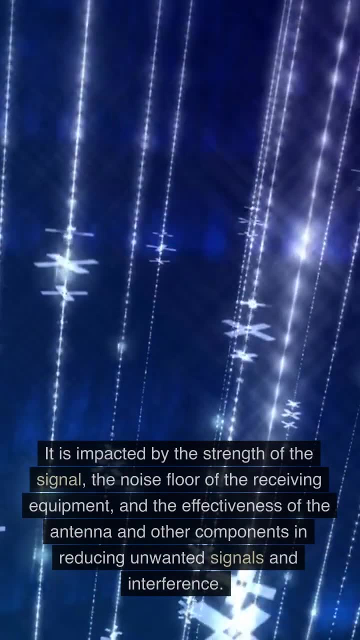 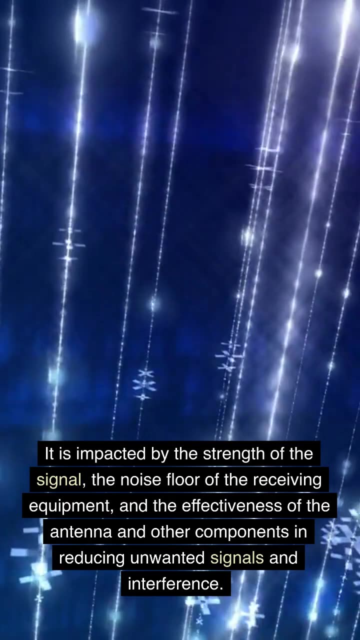 Improving the SNR can help ensure clear and reliable communication, especially in weak signal or long distance situations. It is impacted by the strength of the signal, the noise floor of the receiving equipment and the effectiveness of the antenna and other components in reducing unwanted signals and interference. 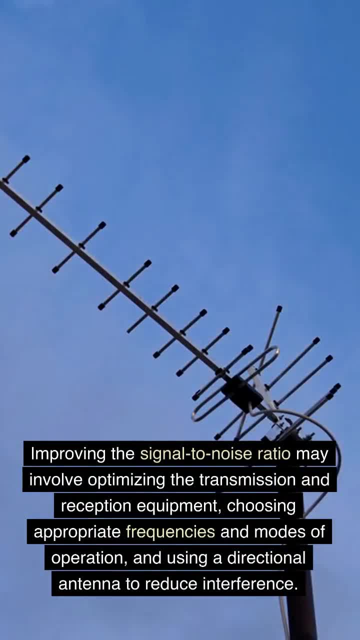 Improving the SNR may involve optimizing the transmission and reception equipment, choosing appropriate frequencies and modes of operation, and using a directional antenna to reduce interference. 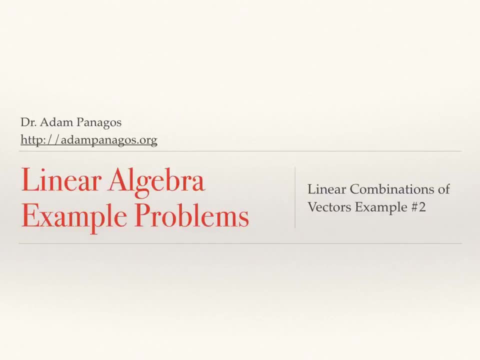 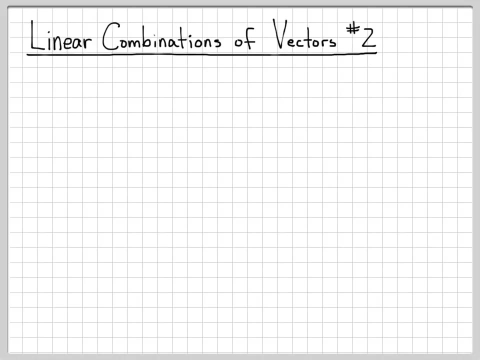 So in this video we're going to again work with vectors and determine if a certain vector is a linear combination of a different collection of vectors. So the vectors we'll work with in this example are x1, x2, and x3.. Here are the three vectors And our question again. 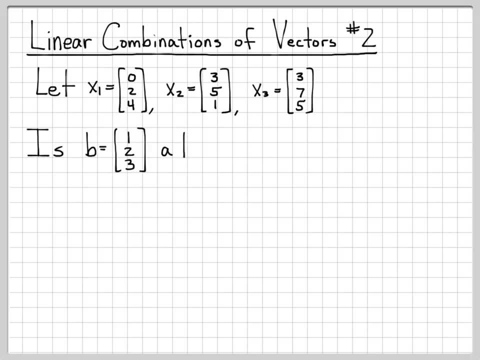 is given this vector b, which is 1,, 2, 3,, is b a linear combination of x1,, x2, and x3? That's our question that we're trying to ask, Mathematically, what that means is: is it? 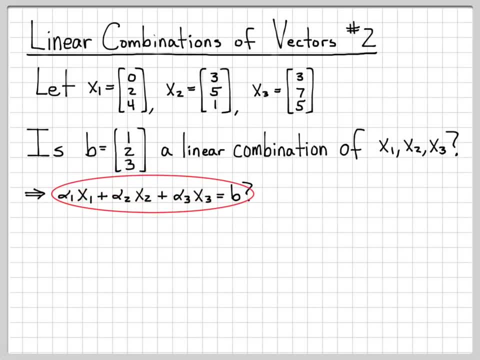 possible to write b as a linear combination of the vectors x1?. So is it possible to find alpha 1,, alpha 2, and alpha 3 to make this equation true. So this is the vector form of the equation that we would like to solve, if possible, for alpha 1,, alpha 2, and alpha. 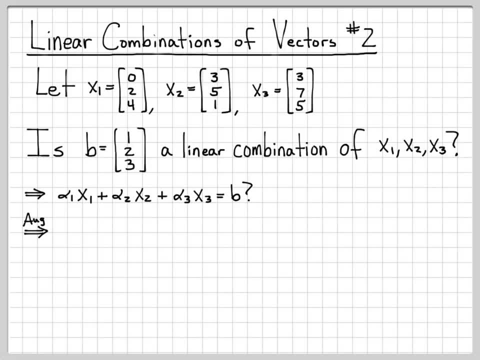 3. Equivalently, I can write that as an augmented matrix. So the augmented matrix has x1 as the first column, x2 as the second column, x3 as the third column, And the vector b forms the fourth column of this augmented 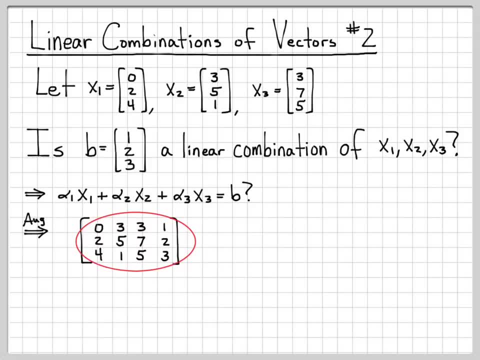 matrix And if I can solve this augmented matrix, it will tell me what alpha 1,, alpha 2, and alpha 3 are In general. solving an augmented matrix means performing elementary row operations to manipulate the augmented matrix into a reduced form or a row-reduced